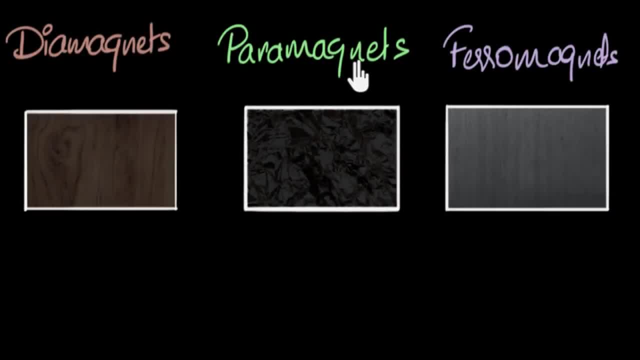 In this video we want to put a number to how diamagnetic or paramagnetic or ferromagnetic things are. For example, if somebody asks how diamagnetic is wood or how paramagnetic is aluminum, how do we provide a number? how do we put a number to that? 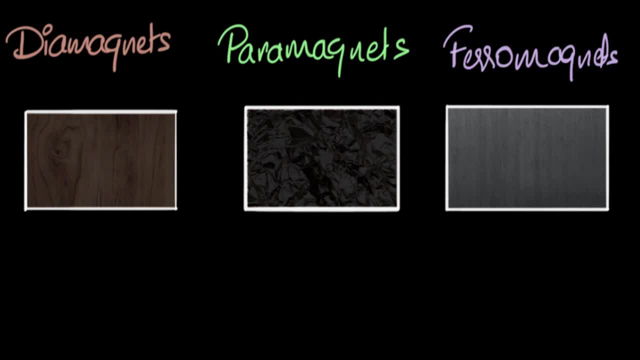 That's what we're gonna explore over here, And we'll start by introducing a uniform magnetic field through all these materials. Imagine there's a giant bar magnet somewhere. Now, we've already seen earlier how different materials react to magnetic fields. So based on that and based on your knowledge, 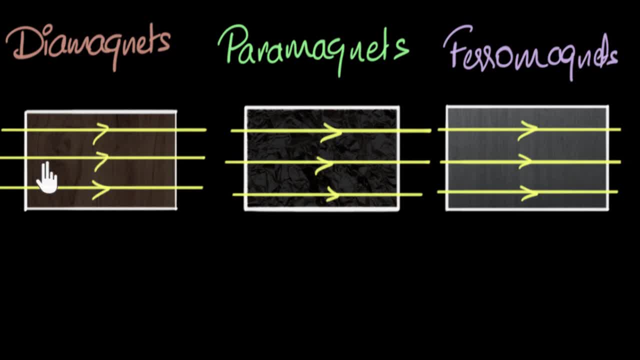 of magnetic field lines. can you predict how the field lines would change inside these materials, How the field lines would be inside wood, How what'll happen to the field lines once it goes through aluminum? What happens to it when it goes through, you know, iron? 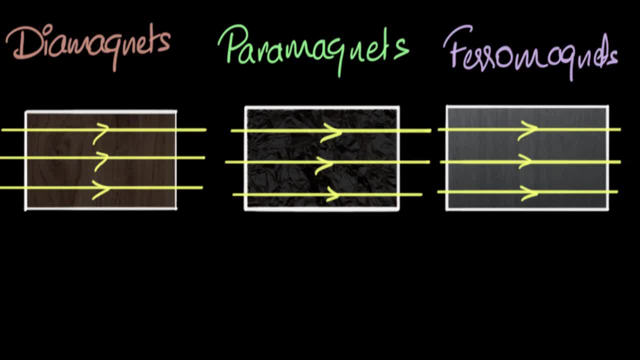 Can you pause and try to predict how the field lines would change inside? Okay, let's start with diamagnets. What is their specialty? They tend to repel magnets right. And how do they do that? Well, they do that by inducing very tiny magnetic moments. 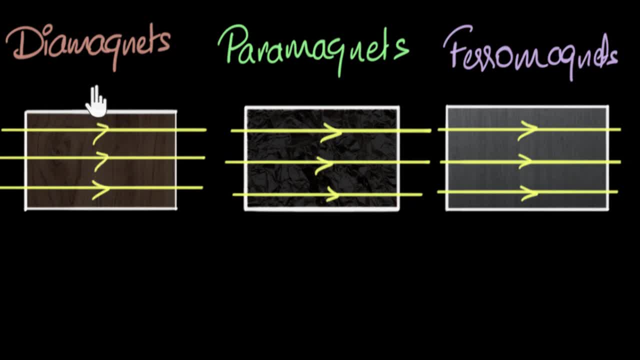 in the opposite direction. Tiny magnets gets induced in the opposite direction And, as a result, there is a very tiny magnetic field induced inside wood in the opposite direction. So let me put that this way: As a result, the total field inside becomes slightly less. 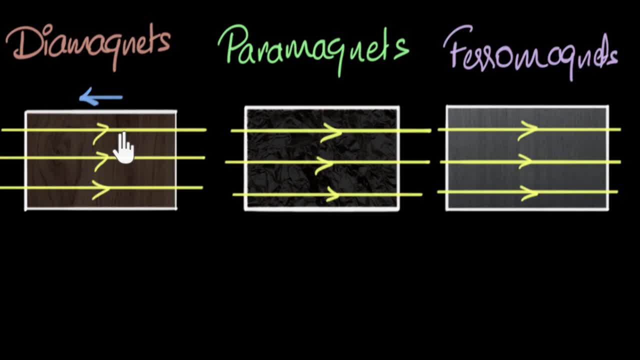 than the field outside. And we've seen in magnetic field lines, if the field value is less, you know the magnetic field lines is less. we like to draw the lines farther away. Okay, so from this, can you pause and now think about? 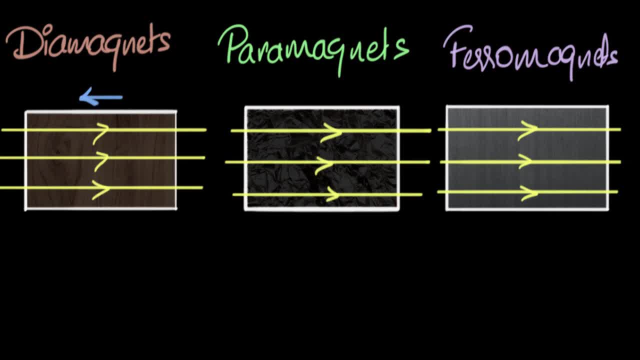 how the field line should look inside a diamagnet. Okay, so the field lines inside should go farther away from each other, so the field lines would look somewhat like this. So you see, diamagnets tend to expel the field lines out of its body. 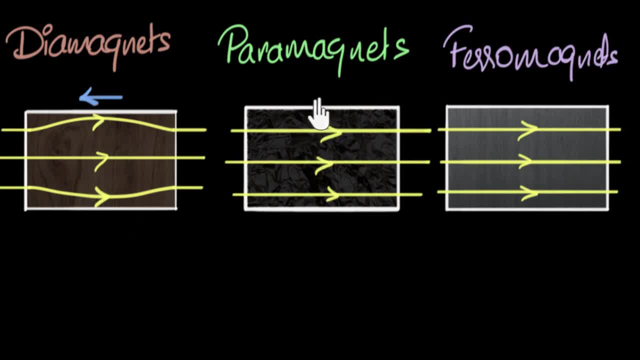 That's a specialty of them. All right. what about paramagnets? We know that these have tiny permanent dipoles. They have tiny magnets inside, but they are all all in random direction and when you put a field, 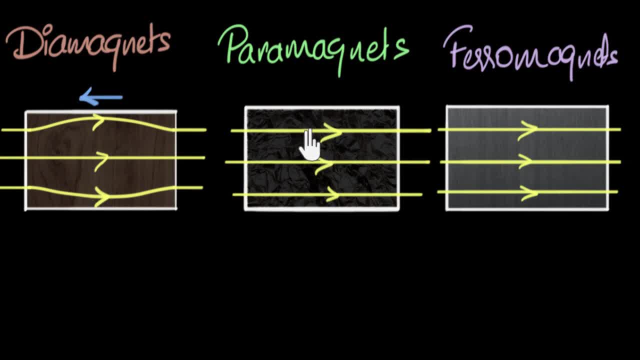 they all get aligned pretty much in the same direction and as a result of that there is a very tiny magnetic field produced in the same direction, which means the total field inside becomes slightly higher than the field outside, because they're induced field and this is in the same direction. 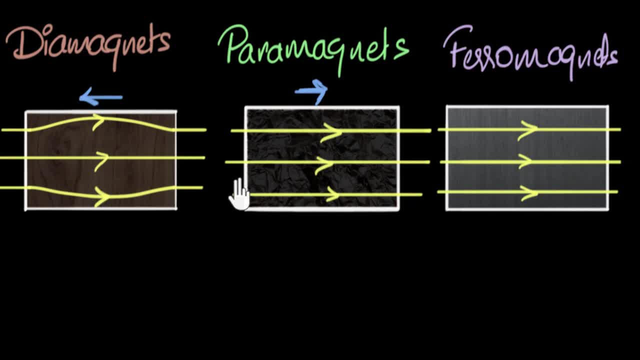 which means the magnetic field lines are slightly closer to each other compared to the outside. So what would that look like? Well, it would look somewhat like this. So you can see, paramagnets tend to kind of suck the magnetic fields towards each other, but very slightly. 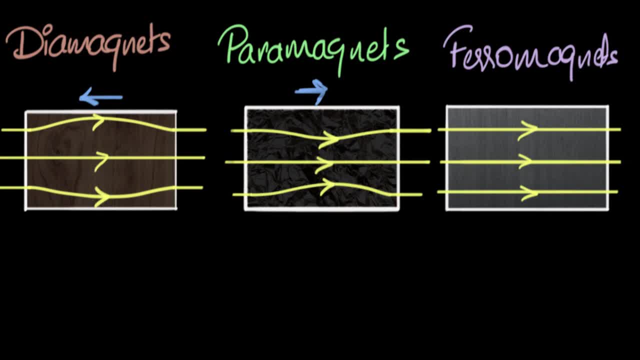 Both these effects are very slight, very tiny. I've exaggerated over here. What about ferromagnets? Well, we've seen that these have domains inside, and when you put an external field, if it's strong enough, the domains turn. you have superb alignment. 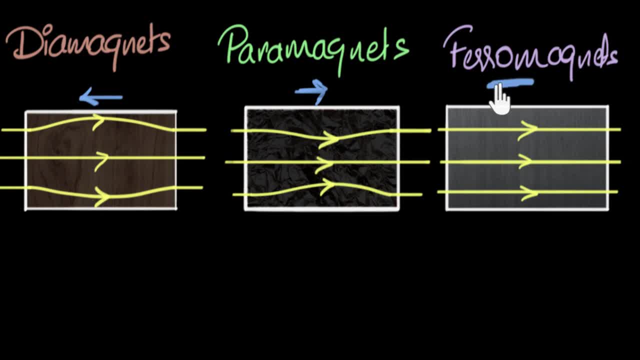 and, as a result, you have an extremely strong magnetic field generated or induced inside. I'm gonna put a thick arrow mark over there. okay, Very strong magnetic field induced and, as a result, the field inside is incredibly strong compared to the outside. 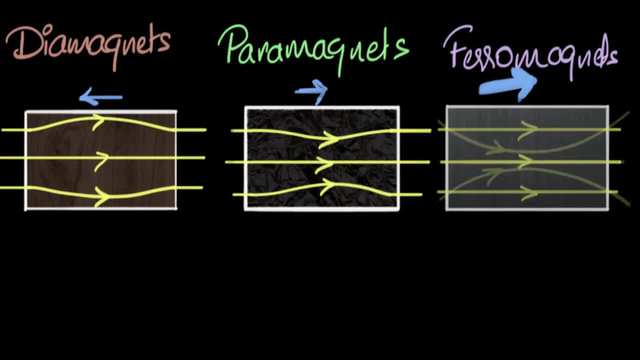 So what would it look like? Well, the field lines would be very, very close to each other, and so you know, this is how we're gonna draw. Again, this is they need to be really, really close compared to the field outside, because it's incredibly strong. 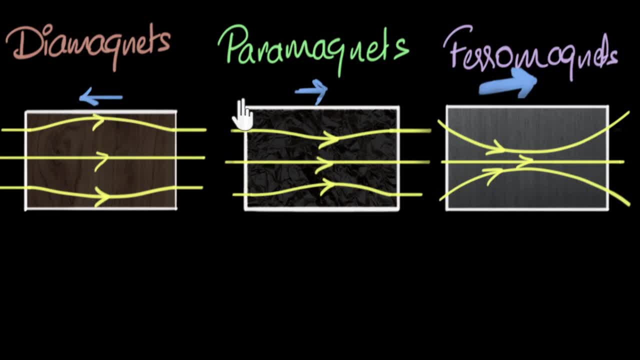 We'll see how strong it is in a while. All right, so to start putting a number to this, we have to build some equations, and for that let's try to label these magnetic field. Now there are multiple fields over here. 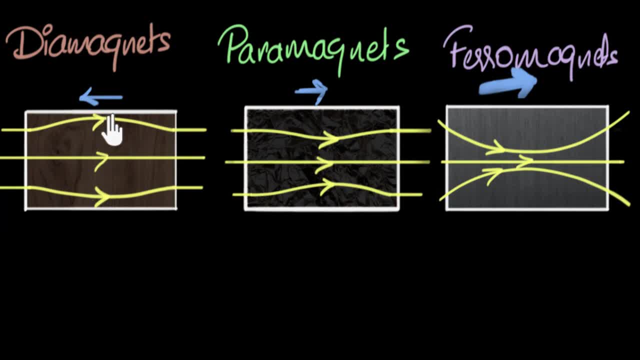 First of all, we have the field which is in vacuum, the field in the absence of, say, the wood or this aluminum. Let's call the vacuum field B naught. So I'm just gonna call that B naught. The vacuum field is B naught. 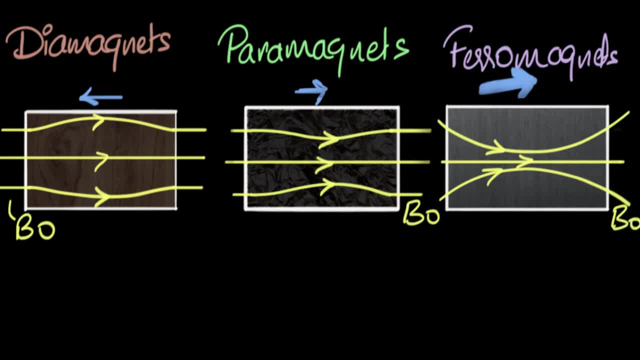 The vacuum field is B naught. Then we have the field that gets induced as the materials react to it. Let's call it as the induced field. B in B induced, let's call that as B induced And then, because of this, the total field inside. 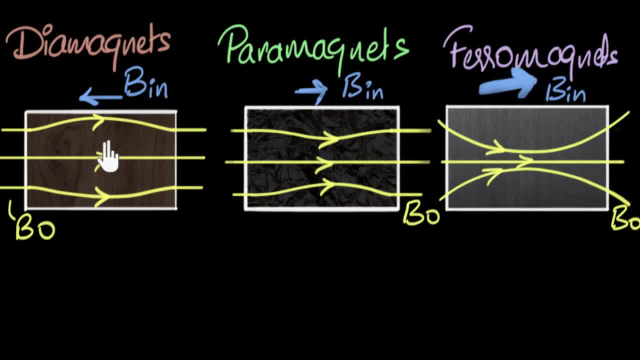 is gonna be a sum of these two. right, It's just gonna be a sum, a vector sum, you can say, And so that total field, the net field inside, is gonna be just B. I'm just gonna call that as B. 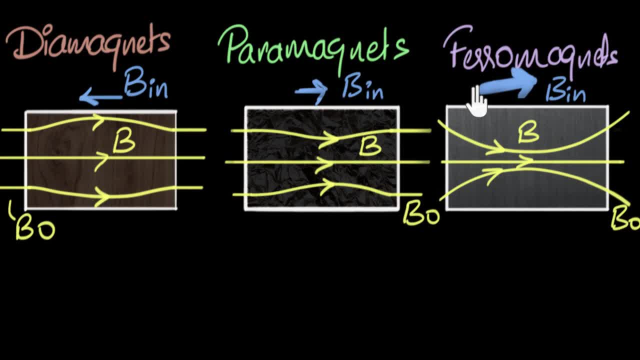 So now, the main question I have is: what does this induced magnetic field depend on? Well, clearly, they depend on the material, whether it's a diamagnet or a ferromagnet, and you know whether we're dealing with copper. or we're dealing with nitrogen- definitely depends on the material, but it also depends upon the strength of the external field, right? I mean, if the external field goes to zero, we've seen that the induced fields go to zero in these cases. 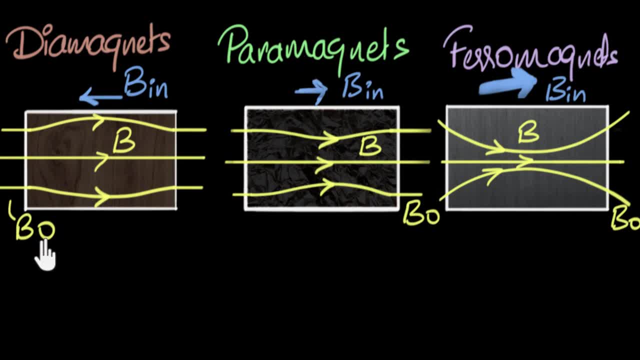 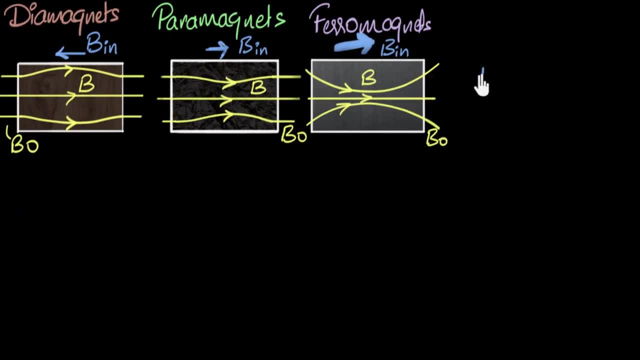 They are temporary. They are temporary effects. On the other hand, if the external field gets stronger, we would expect the induced field also to become stronger. So it turns out to some degree of accuracy we can write that the induced magnetic field 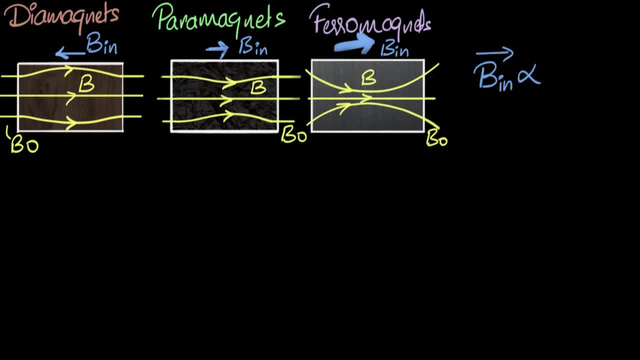 and I'm writing it as a vector- is proportional to the external, the vacuum field, And whenever there's a proportionality sign, we can always replace it with an equal to and a constant, and that constant is often called xi or qi, I think. 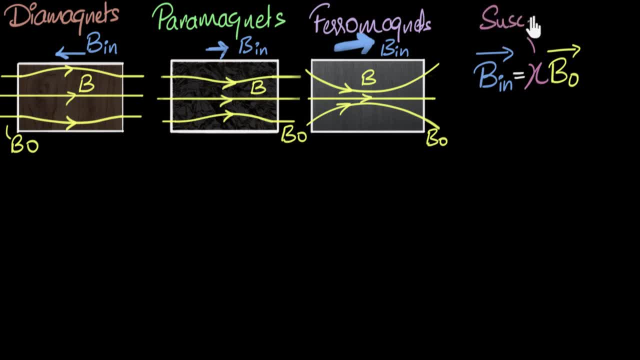 one of them, and it's called susceptibility, magnetic susceptibility. And what does this constant tell us? Well, let's see, Let's put some number. If we put this zero, then that means that the induced field would always be zero. 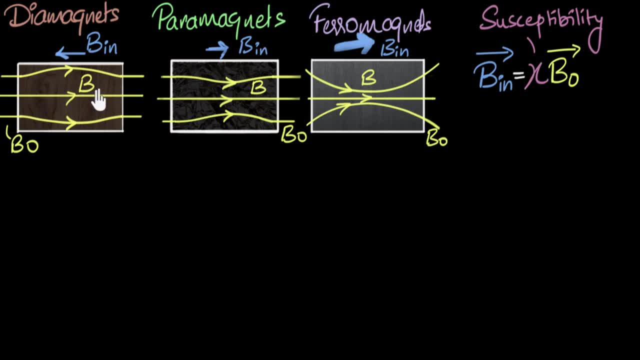 There'll be no magnetization at all. It wouldn't react to the magnetic field at all. On the other hand, if the susceptibility value is very high, that means you have a strong induced field. Very nicely, very vigorously, it reacts to the external field. 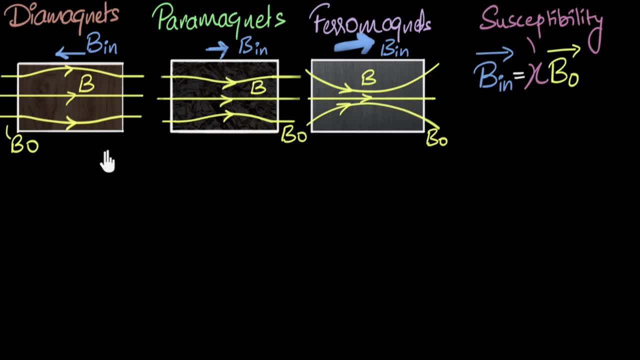 So, hey, this number directly tells us how readily materials can get magnetized when you have an external field. So this is the number that we're looking for And that's why it's called magnetic susceptibility, because it tells you how susceptible or how readily materials can get magnetized. 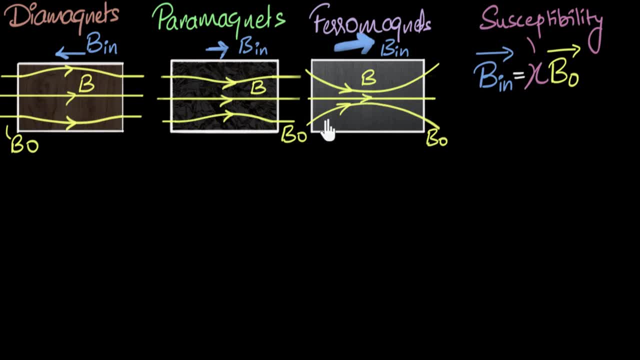 Now, before we start looking at the values of susceptibility of different common materials, I want you to make a prediction again. I want you to think about whether the susceptibility values would be very high or low for these materials And also think about: would they be a positive number? 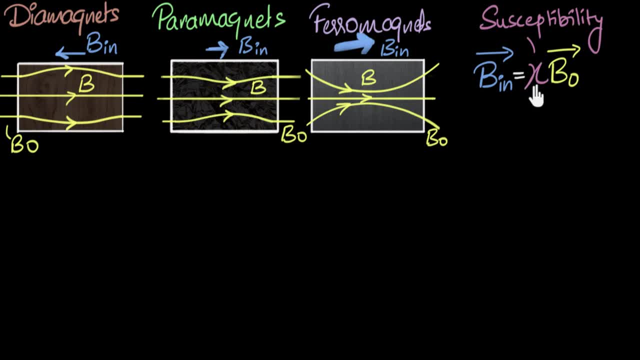 or a negative number for these materials. What would be the unit of this Think about? can you ponder upon all of this before we start looking at the values? Then the values will make a lot of sense there. All right, let's see. 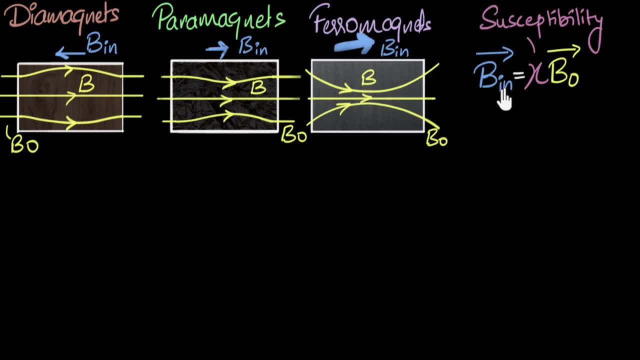 First of all, let's look at the units. Both of these are magnetic fields, right? So the units should be nothing. They should be a unit-less number, dimensionless number. Okay, what about its value for diamagnets? First of all, would it be a high value or a low value? 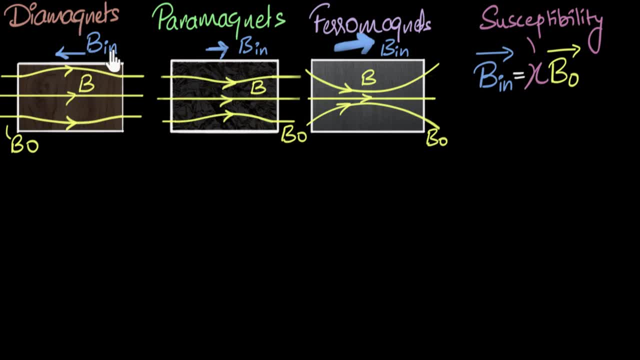 Well, we know, diamagnetism is a very, very weak phenomena. That means the induced field is gonna be very tiny, very, very tiny compared to the external field, and so we would expect this number to be very, very tiny. Lastly, would it be a positive number or a negative number? 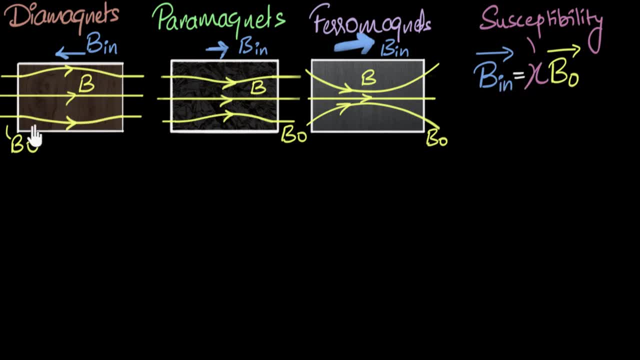 Well, for that, think about the direction of the induced and the external field. Well, if the external field is to the right, then the induced field is to the left because diamagnets, you know, they tend to repel the field right. 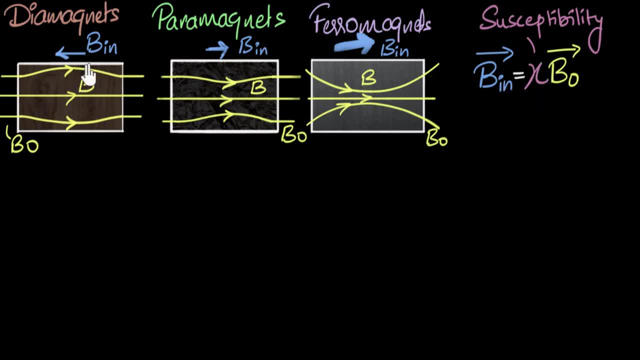 Ooh, this means the susceptibility value for diamagnets should be negative, it should be very tiny and of course it should be dimensionless. So let's look at some numbers and see if that makes sense. So it turns out. susceptibility values for copper and water. 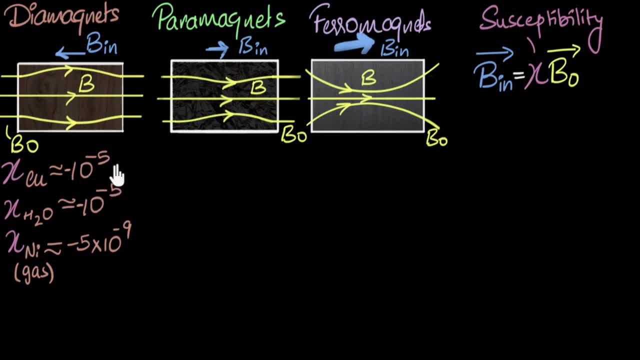 is very similar- about minus 10- to the power minus five. Look at how small it is. Exactly what we predicted: negative. exactly what we predicted: no units. We'll look at the susceptibility of nitrogen gas. It's way way smaller, mainly because it's a gas. 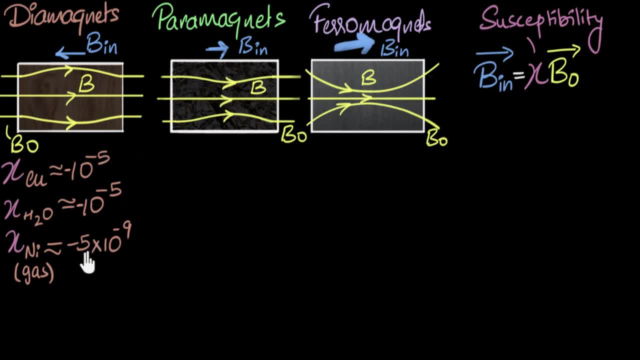 so less number of atoms, less induction and, as a result, smaller induced field, smaller value of G. And, by the way, we don't have to remember any of these numbers. What about paramagnets? Well, again, there's a very weak phenomena. 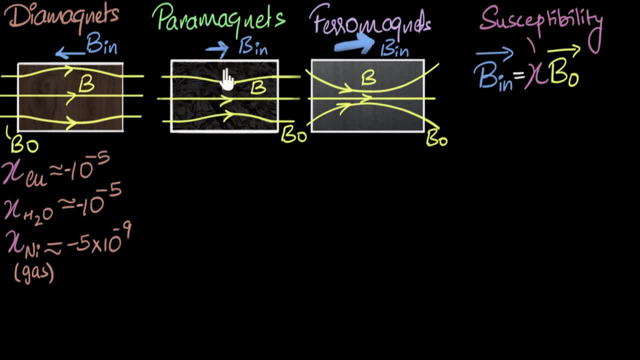 so we would expect you know G value, or susceptibility value, to be very tiny, something similar And it's- do you think it's positive or negative? Well, over here, they induce field in the same direction as the external field, so we'd expect them to be positive. 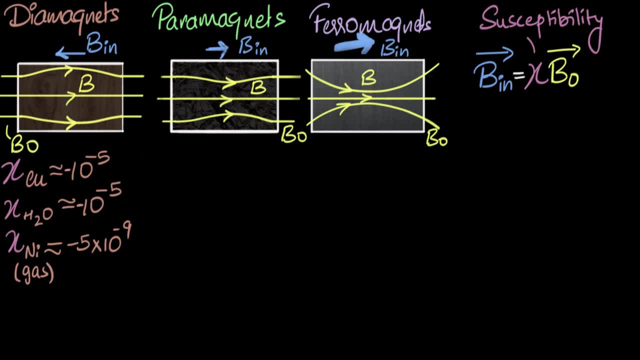 So tiny, so positive, small numbers for paramagnets. So let's see, let's look at some values And we get small numbers and we get positive numbers. Yay, that's nice. So for aluminum it turns out to be: 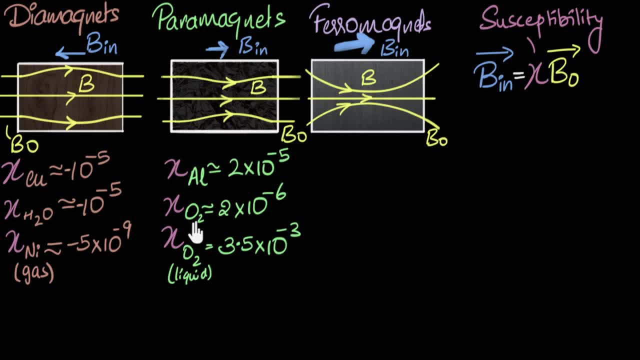 about two times 10 to the power minus five. Look at for oxygen gas. This is oxygen gas: about two times 10 to the power minus six. But look at liquid oxygen: 3.5 times 10 to the power minus three. much higher. 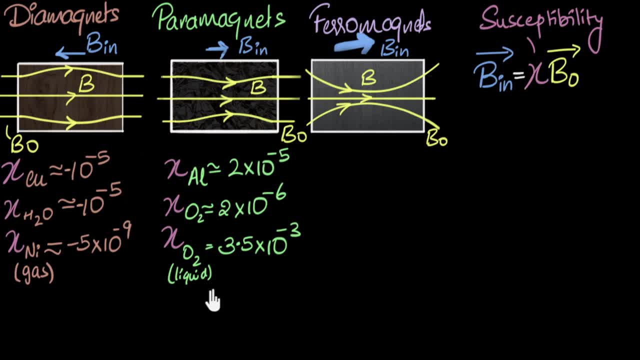 Why is it much higher for liquid oxygen, Something we've seen before? Ooh, that's because paramagnetism depends on temperature. Lower the temperature, easier it is to align these dipoles inside and, as a result, stronger paramagnetism. 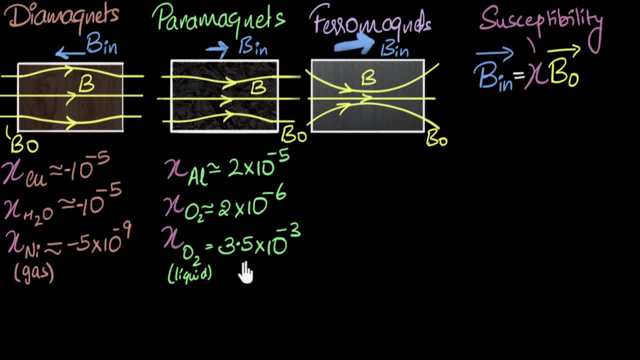 And we've talked a lot about this in previous videos, videos on, you know, videos on paramagnets and diamagnets, So feel free to go back and watch that if you need a refresher. But when it comes to diamagnetism, 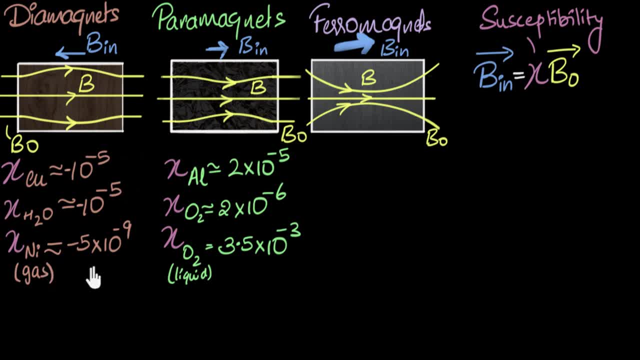 it really, really doesn't depend too much on the temperature, So you would get pretty much the same value or similar value for nitrogen liquid. Okay, what about ferromagnets Now? to be very precise, there is no direct relationship between the induced field and the external field. 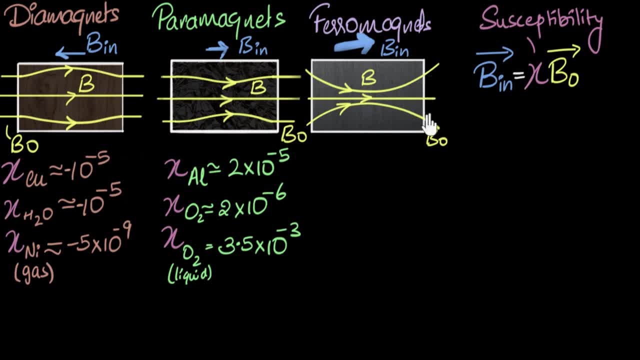 And you know we'll talk about that in a separate video when we talk about hysteria- Hysteresis, But we can give some ballpark number connecting these two. We know that the induced field inside is gonna be much, much higher than the external field. 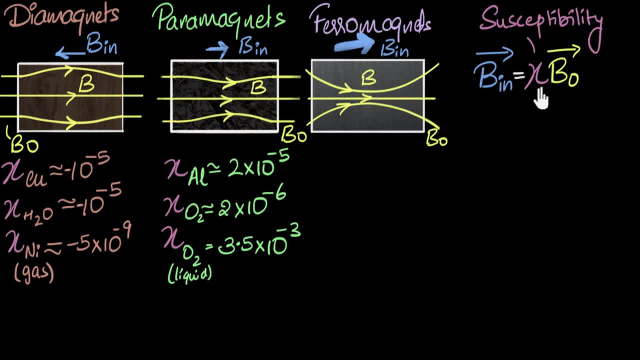 And it's gonna be in the same direction. So you would expect susceptibility to be incredibly high number and it's gonna be positive. So it turns out. the numbers can be somewhere between 100 to about 10,000, or even a million. 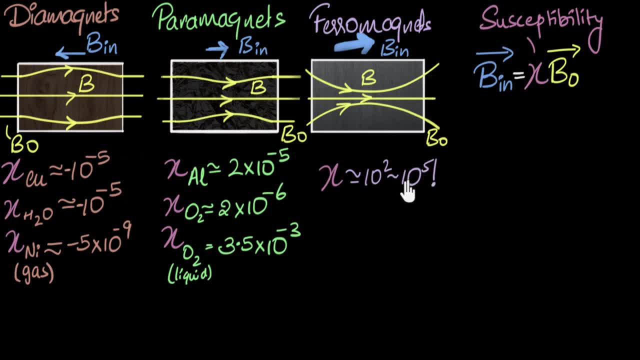 Ion, for example. I just looked up it turns out to have susceptibility about 200,000.. That's ridiculously high value. Now, before we move on to the last part, this quick disclaimer. if you look into your textbooks or some online resources, you will find. 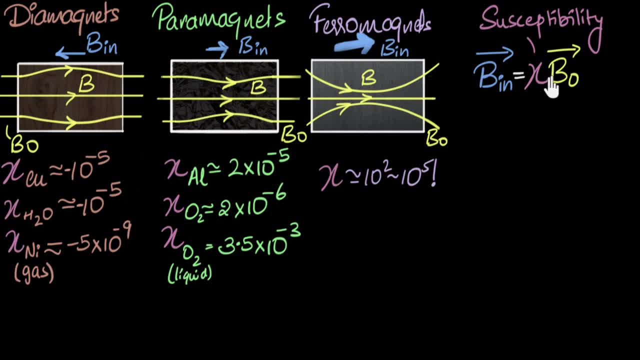 this is not how susceptibility is formally defined. It is usually defined in terms of a vector called magnetization and magnetic intensity. But to understand the meaning of susceptibility, we don't need to introduce those terms, and that's why I like to at least introduce them. 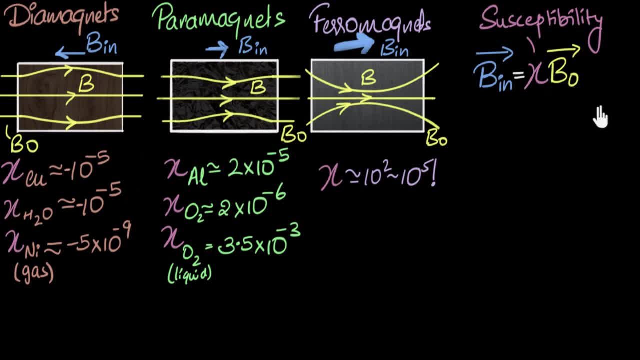 in terms of normal magnetization, Normal magnetic field that we are familiar with. Maybe in future videos we'll introduce those new terms as well, But the last thing we're gonna do is find an expression, write an expression for the total magnetic field. 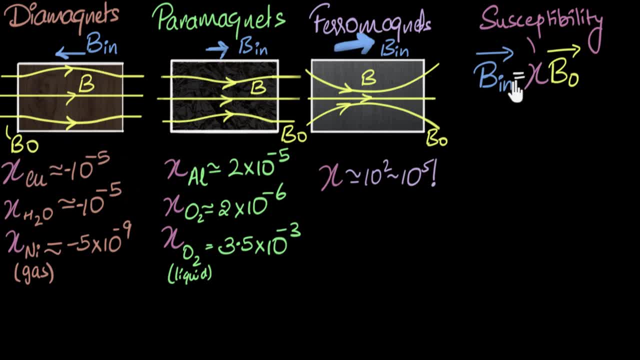 which is just the sum of the external field and the induced field. So again, can you pause and see if you can go ahead and write that equation? Okay, let's do this. So the total field inside is just gonna be the sum of the vacuum field and the induced field. 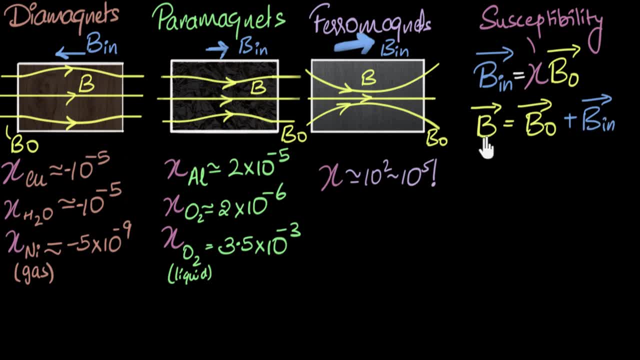 If there was no material, then the induced field would be zero and the total field would be just the vacuum field. Makes sense, right? And we now know that the induced field can be written as the susceptibility times. the vacuum field And therefore the total field inside is just gonna be. 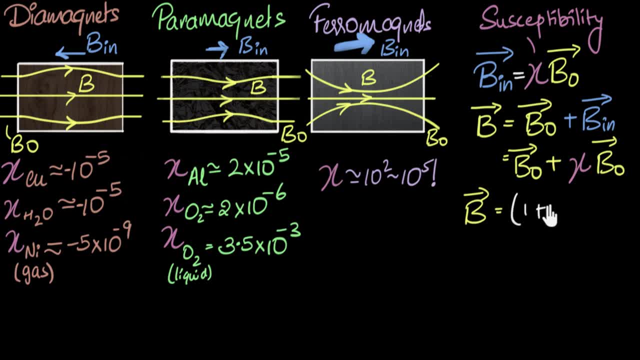 one plus the susceptibility, one plus the susceptibility times, the vacuum field. And because this relationship is pretty useful for us, because most of the time we are interested in what the total field is inside a material, we like to give this one plus chi another name. 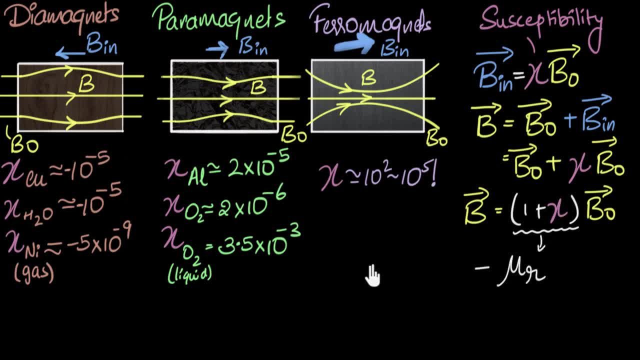 We call that mu r And that's called the relative permeability. Permeability And that is just one plus this number, And because diamagnets and paramagnets have very tiny values of chi, that basically means this number is pretty much gonna be one. 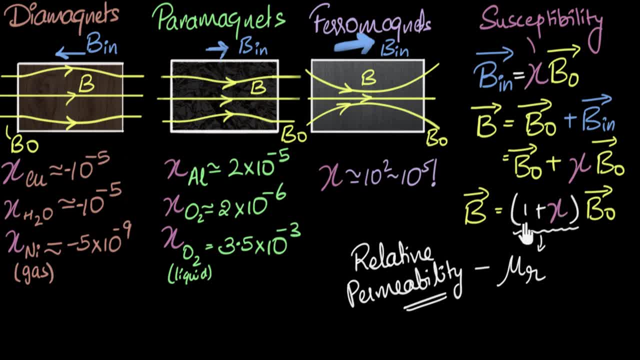 For diamagnets it's gonna be slightly smaller than one. It's gonna be one minus 10 to the power, minus five Slightly. it's gonna be 0.999 something. For paramagnets. it's gonna be slightly higher than one. 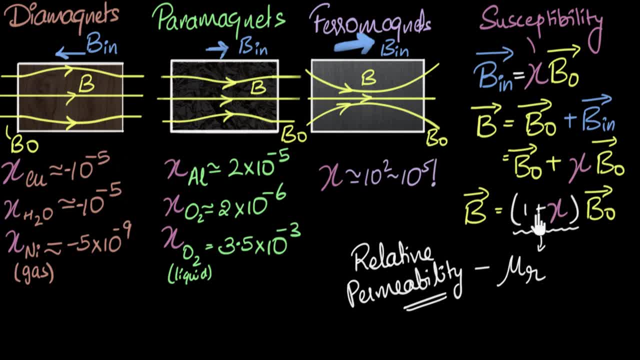 One plus two times 10 to the power minus five is 1.000 something. But for ferromagnets, oh, It's gonna be. these values are pretty much comparable. Mu r value is also gonna be 10,000, 100,000, a million. 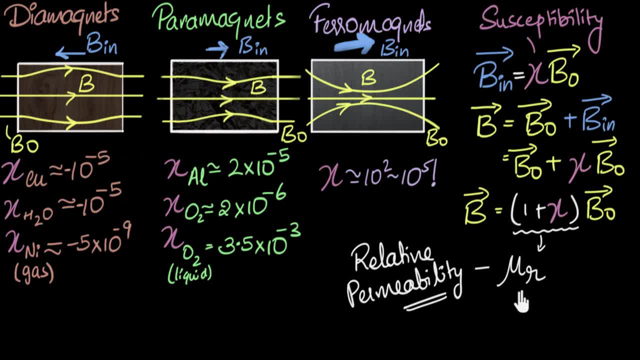 So the magnetic field inside any material is just gonna be mu r, the relative permeability times the magnetic field, the vacuum field. All right, before we leave, I want to give you a fun fact. There are certain diamagnets and I won't tell you which one. 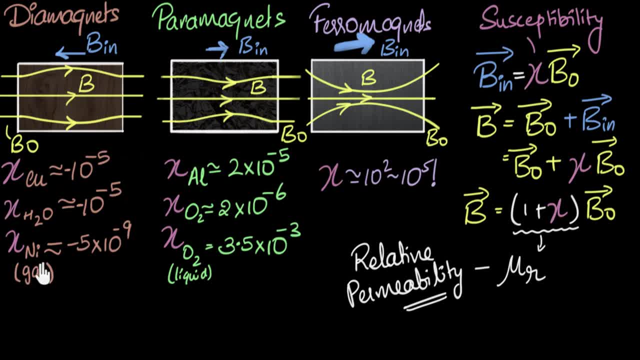 I want you to do the research. They have chi value to be negative one. They're called perfect diamagnets. I want you to ponder upon that. Why do we? what does it mean to have negative one? What would happen to their permeability? 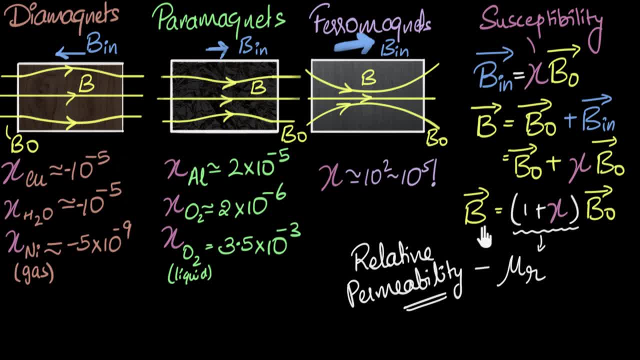 What would be the magnetic field inside? What's the implication of that, Do you know? And which materials are these? I want you to do some research around that.